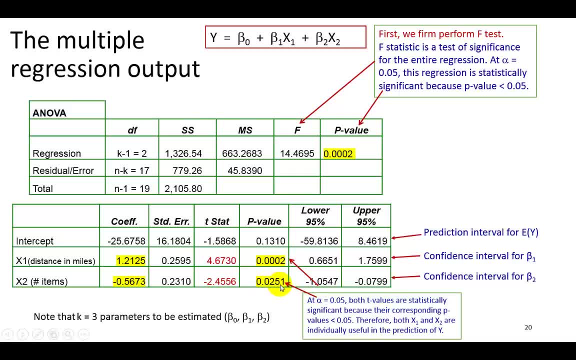 At the 5% level, distance in miles is significant. At the 5% level, number of items contained in each package is also significant. So at the 5% level, both are statistically significant and we're quite happy with that. 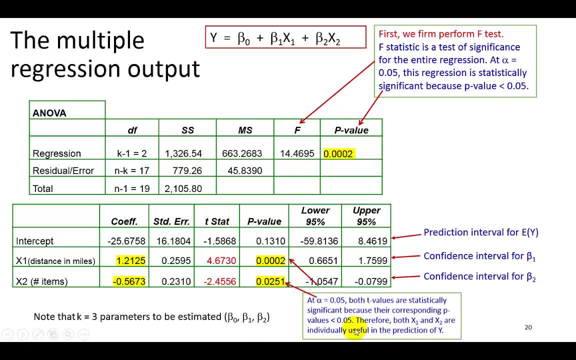 So we can therefore conclude that both X1 and X2 are individually useful in the prediction of Y, the cost of shipment. So to wrap this up: first, the regression as a whole is statistically significant and that's based on the F statistic. 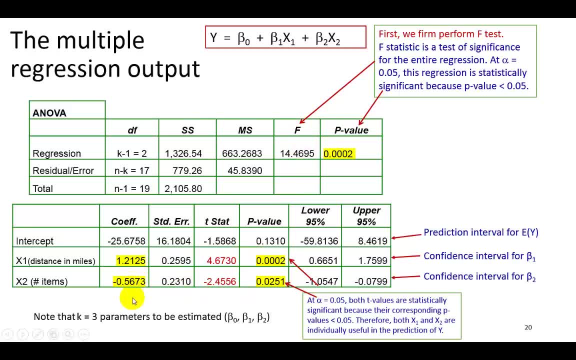 And secondly, the individual coefficients tell us that, individually, each of these variables contributes meaningful information in the prediction of Y. Now, what you see here is a 95% prediction interval for the mean value of Y, which is in the case where X1 and X2 are 0, because that's right next to intercept. 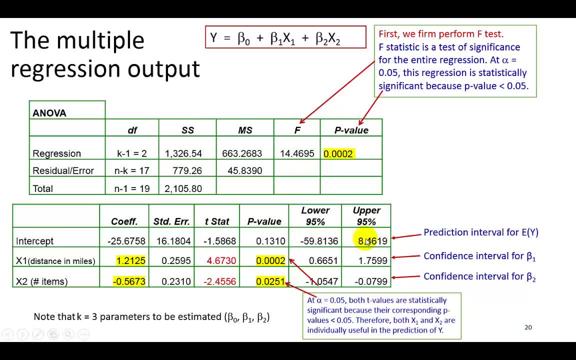 And this doesn't really have much to do with Y, And this doesn't really have much as far as adding spunk and substance to multiple regression is concerned. You might, however, be interested in knowing what the 95% confidence limits are for B1.. 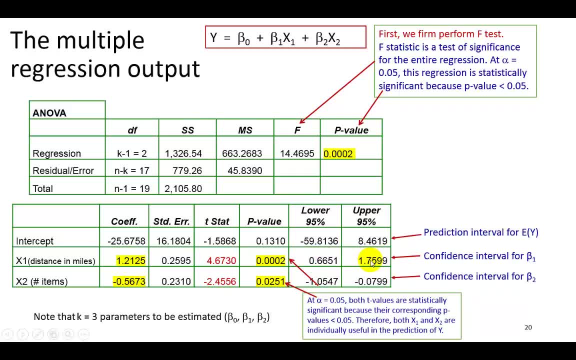 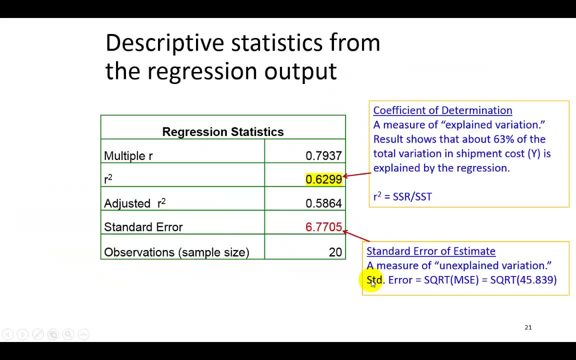 This is the estimate and these are the lower and upper limits. And for X2, this is also the 95% confidence limit, The lower limit and the upper limit. So now the descriptive statistics are summarized here. Importantly, we have R2, which is the coefficient of determination. 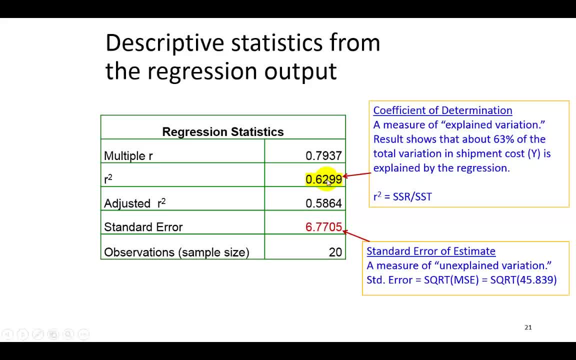 and measures the proportion of the variation in Y that has been explained by the regression And it's calculated as the ratio of the sum of squares regression and the sum of squares total. And it tells us that about 63% of the total variation in shipment cost Y has been explained by the regression. 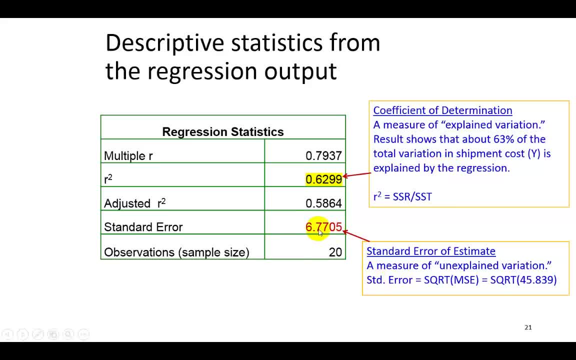 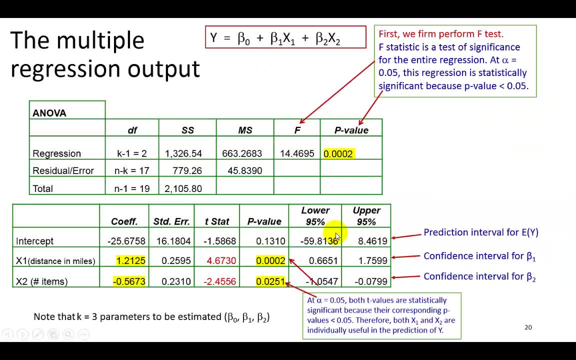 And we have standard error of the estimate, which is a measure of unexplained variation. It is the square roots of the mean square error. If I go back here, the mean square error is shown right here: 45.839.. If you take the square root of this value, as I show right here, 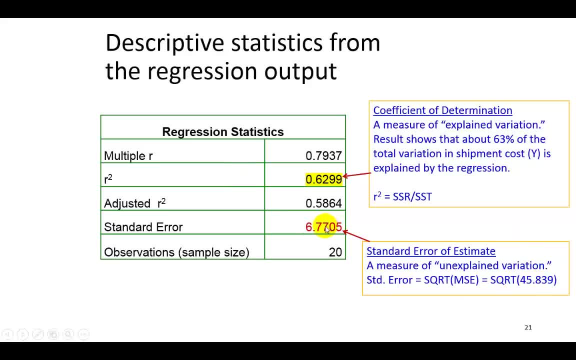 you will find the standard error of the estimate. It's an absolute measure of variation. The larger it is, the more the unexplained variation that you have, unlike R2, which is a percentage measure And, as you're going to learn as you increase, the number of independent variables in a multiple regression model. 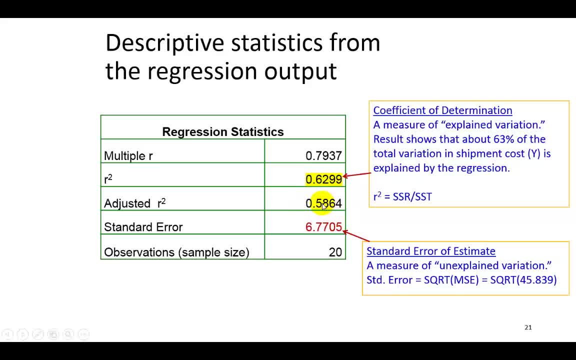 it actually would be more helpful to use adjusted R2 as the indicator for the proportion of explained variation. And the reason explained elsewhere is because, as you add in independent variables, you also you will be increasing R2 ordinarily because you're naturally adding more information into the model. 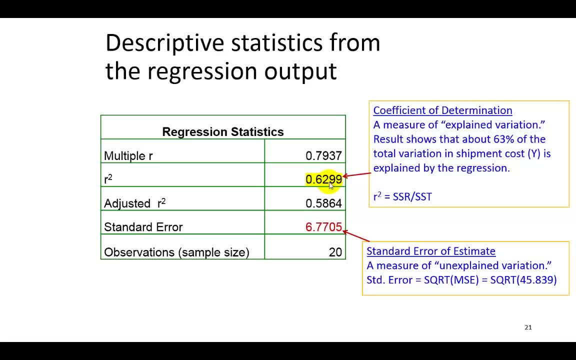 However, you lose degrees of freedom. So the balancing acts between the positive and the negative when you're adding additional explanatory variables as you're adjusted R2.. So this should be more helpful when you have more than a couple of individuals with independent variables in a regression model. 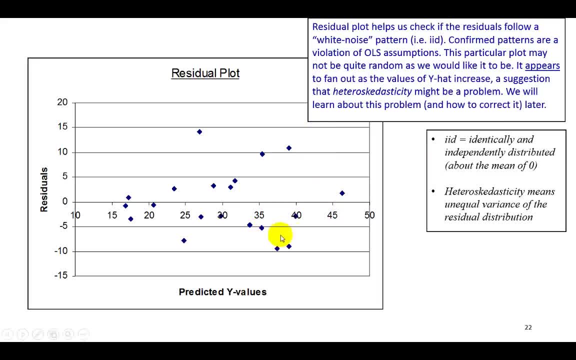 And then we plot the residuals, because residual plot offers us a casual, albeit pretty helpful way of determining if, in fact, the residuals of the model follow a white noise pattern which, if it does, we say that they are identically and independently distributed above the mean of zero IID. 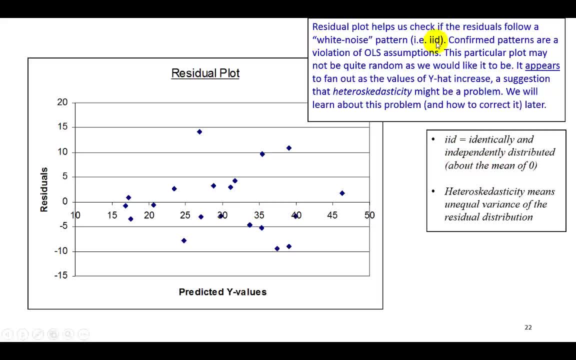 I wrote it out here for you Because we do want it to be white noise, because when it is white noise, then it confirms that the assumptions used in the least squares method have been met. for the most part, White noise means you've expunged all the good information from the data. 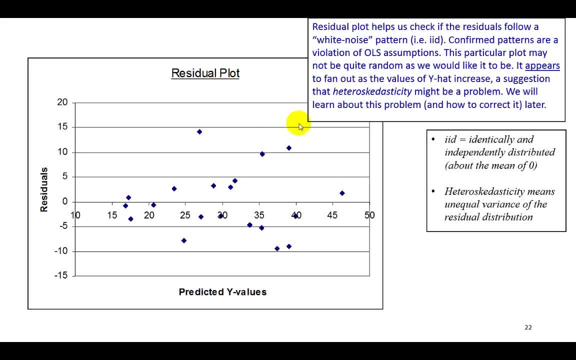 and what's left is just chaff. Now, I observe here, though, that this particular plot may not be quite random as we would like it to be, because it appears to fan out as the values of y-hat increase. As you can see, as the values of y-hat, the predicted values increase. 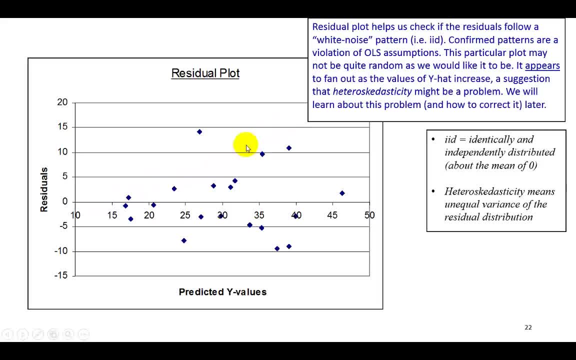 as we go from left to right, you see that there appears to be some kind of a fanning out alright like that. So this is telling us that we may have a problem called heteroscedasticity, which means unequal variance. 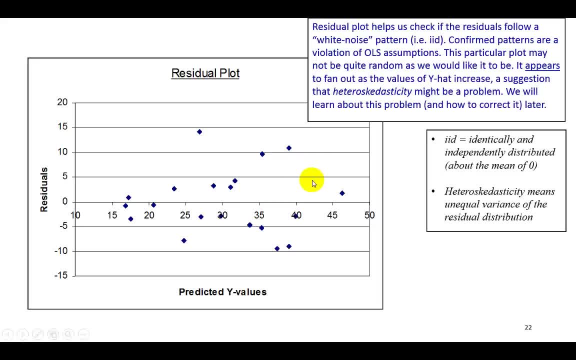 We do want our variance to be equal, which means we do want our variance to be the variance of the residuals to be homoscedastic. We're going to learn more about this in subsequent presentations. In any event, that's what we got right here. 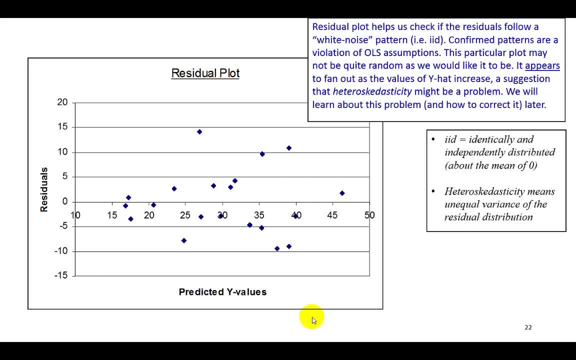 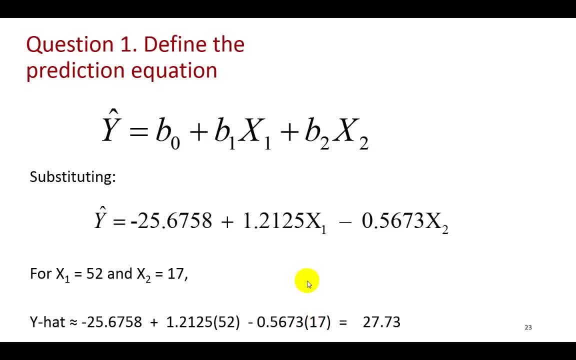 when we plot the residuals of the model, which I showed you how to obtain, those from the regression study in the previous video, A couple of Q&As. It says: define the prediction equation. that's it right here, with the substitutions shown here. 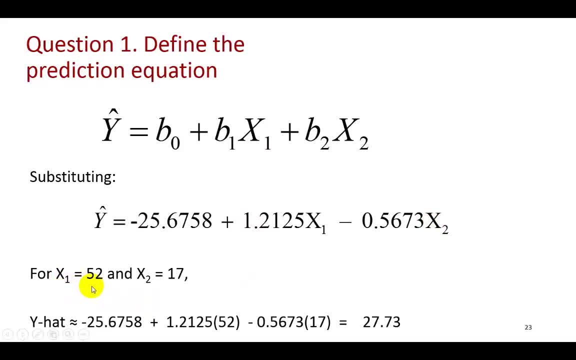 And an example of prediction right here: if x1 is 52 and x2 is 17,, you plug and play and you find your y to be 27.73.. Next up, it says what proportion of the total variation in the cost of shipment. 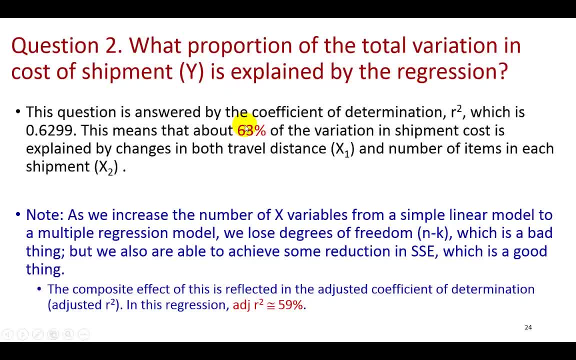 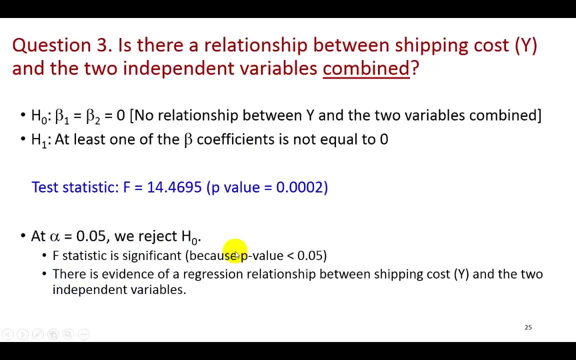 is explained by the regression. We've already addressed that. It's about 63%. That's your coefficient of determination, And the helpful information that you might get by using adjusted R-square is summarized right here. And then question three says: is there a relationship between y the shipping cost? 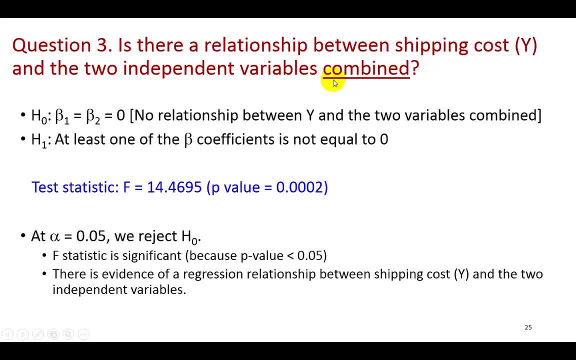 and the two independent variables combined. Now this is the statement of hypothesis, which is that the coefficients are all equal to zero. The alternative has to be worded because this is a multiple test right here. So the alternative hypothesis is that at least one of the beta coefficients is not equal to zero. 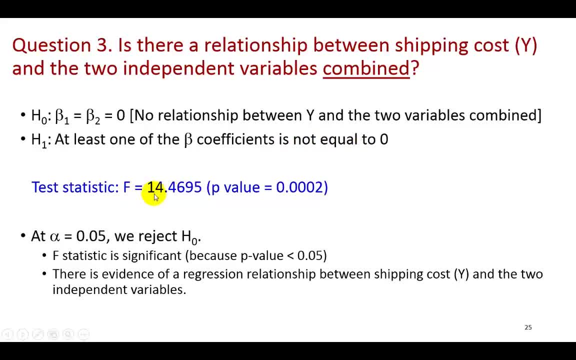 And from the results, we find the F-statistic to be 14.47, with a p-factor. So 14.47 with a p-value of virtually zero, telling us that we must reject the null hypothesis and conclude that a regression relationship does in fact exist. 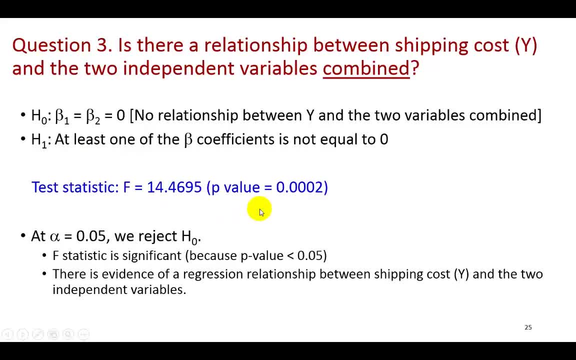 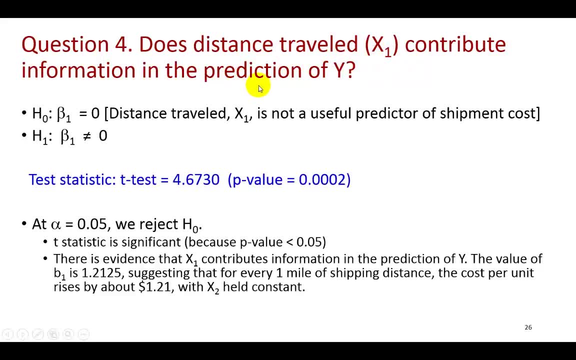 at any conventional level of significance. Question four says: now: does distance traveled, which is x1,, contribute information in the prediction of y? Now, for this we're testing solely the coefficient of x1, which is b1. So this is a unique test. 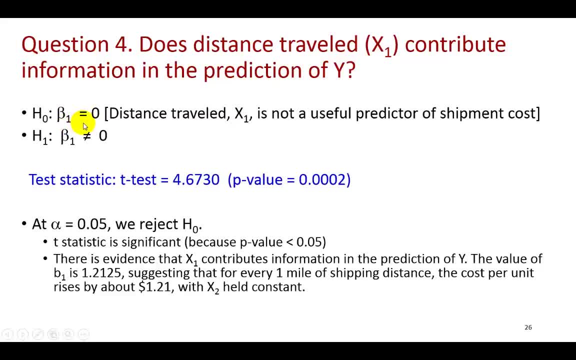 and it's going to be a t-test, And the t-statistic we found is 4.67, with a p-value that's virtually zero, telling us that at any conventional level, we must reject the null hypothesis and conclude that distance traveled does provide useful information. 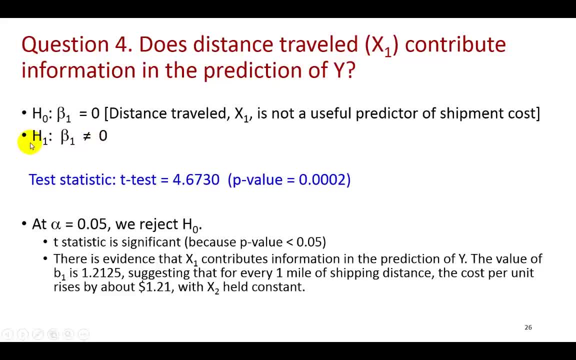 in the prediction of y, in that we have to go with the alternative that now b1 is not equal to zero. So we're quite happy with that, And this is all summarized here. Now notice that the value of b1 is 1.2125,. 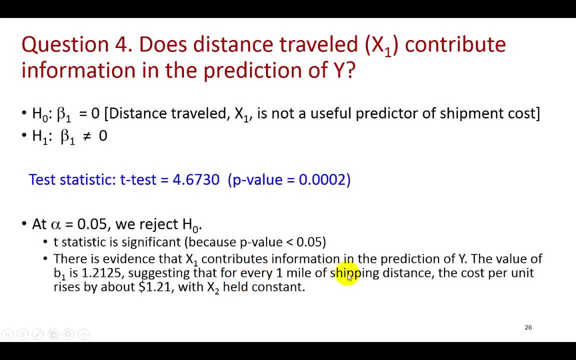 which suggests that for every one mile of shipping distance- since x1 is shipping distance- the cost per unit rises by approximately $1.21, with x2 held constant. We have to remark this because we are trying to identify the unique impact, the specific impact x1 has on y, with x2 under control. 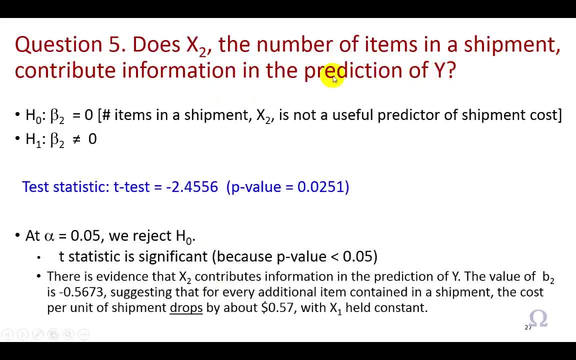 And finally, does x2, the number of items in a shipment, contribute information in the prediction of y? And again, this is a unique test of hypothesis for the coefficient of x2, which is b2.. And we find from the t-statistic next to this coefficient, 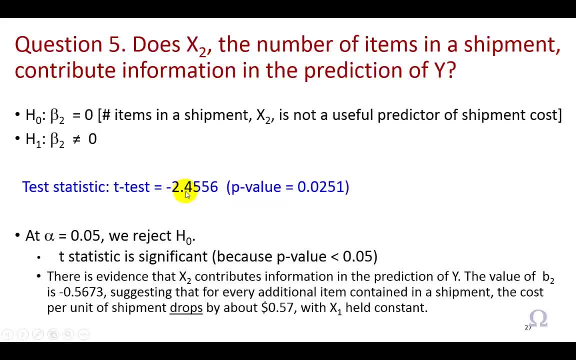 that its value is negative, 2.4556, with a p-value of 0.025, which, at the 5% level, we must reject this null hypothesis and conclude that, yeah, x2 does contribute information in the prediction of y. 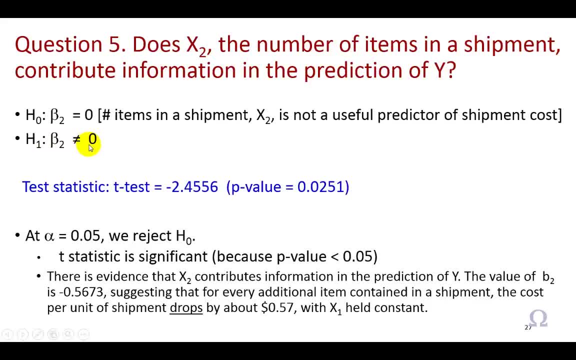 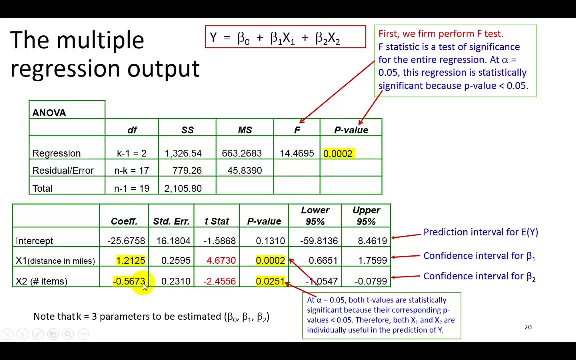 And so we're going with the alternative. Now the results show that the value for b2 is a negative 0.5673.. So if I go right back here, you see it right here. All right, so it's a negative value. 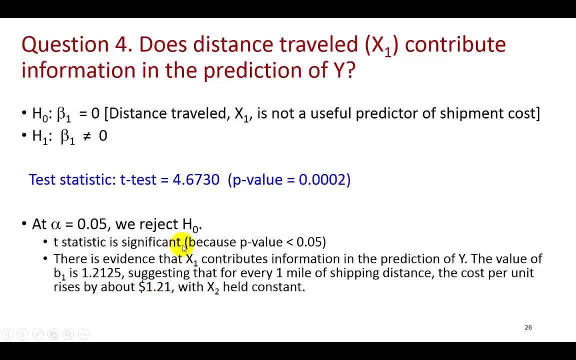 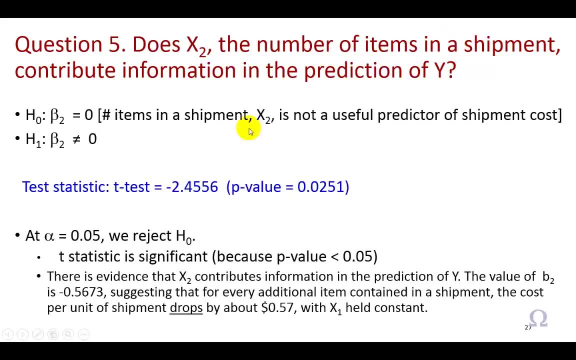 But now bear in mind that x2 is the number of items in a shipment. So what this is telling us, therefore, is that every additional item contained in a shipment, for every additional item in the shipment, the cost per unit drops by about 57 cents.